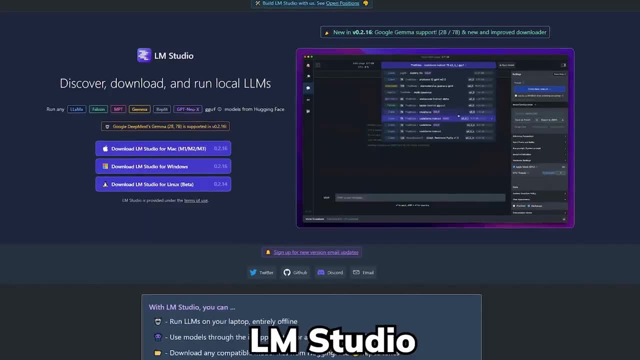 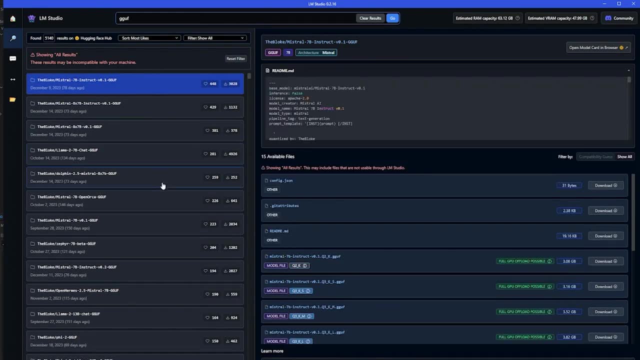 But if you just want some straightforward EXE file, then there is LLM Studio which has lots of great native functions like Hugging Face Model Browser, which makes finding models much more easier. Other than that, it has some much nicer quality of life info that would tell you if you. 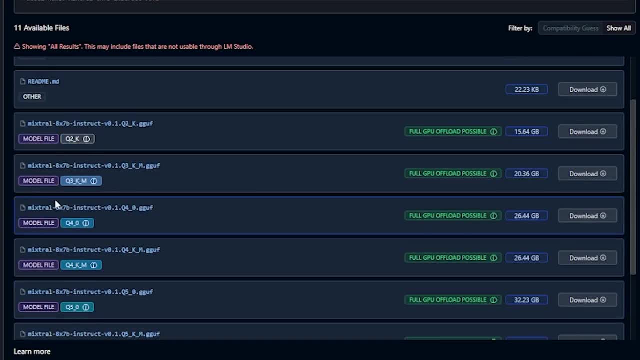 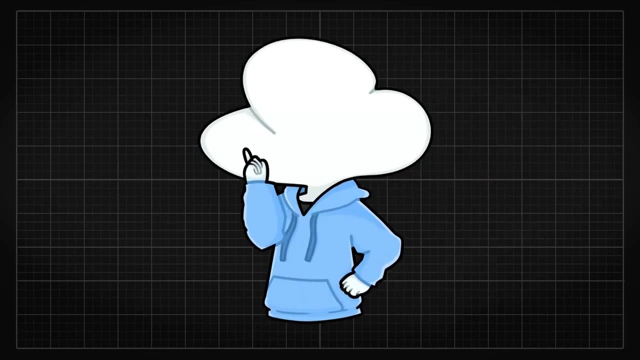 can run a model or not. It's definitely a good alternative. if you don't like the Gradio type of interface, You can hop between models swiftly and you can use it as an API for other apps too. Next we have Axolotl, and it is a command line interface that offers the best support for fine. 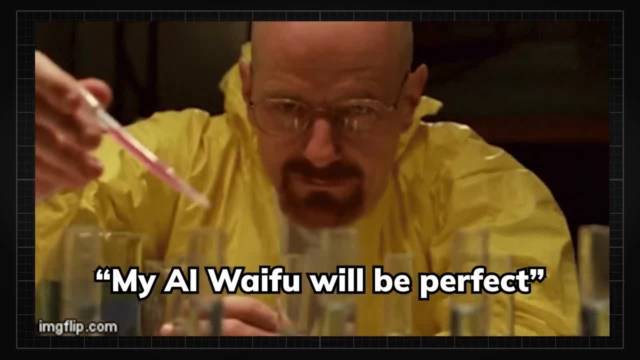 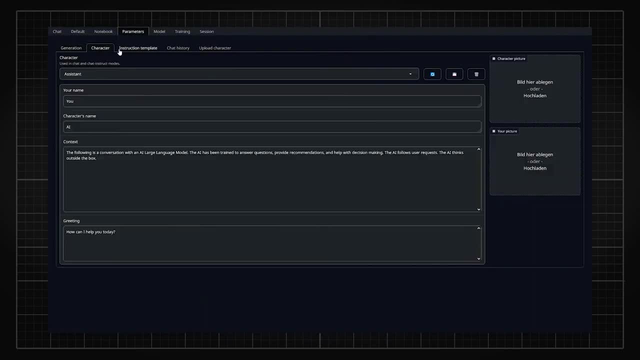 tuning AI models. So if you do get deep into fine tuning, this is definitely your first choice rather than doing it on Ooba Booga. For this video, I will be using Ooba Booga, as it provides the most well-rounded functionalities, with support on most operating systems and available for 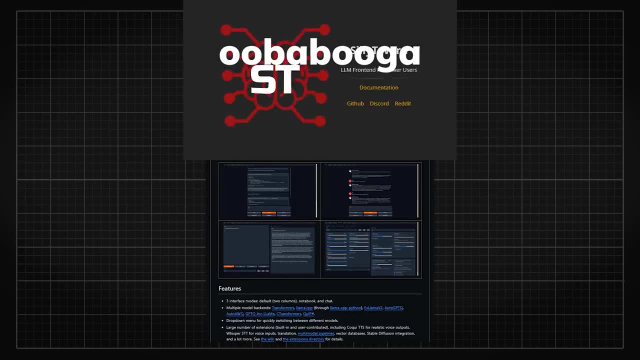 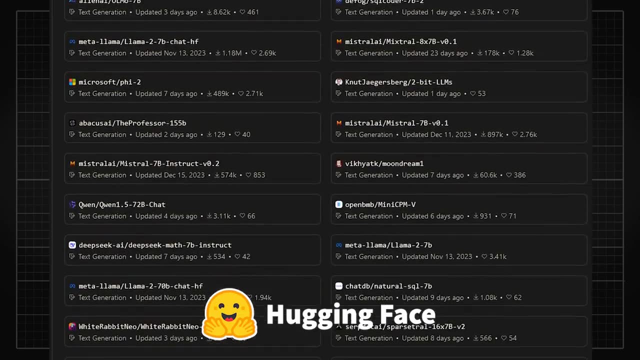 Nvidia, AMD and Apple M series. You can also add silly tarvern as the front end, if you want, And follow these installation steps and you're good to go. Next, you can start browsing all the free and open source models on Hugging Face and download what you want to use using Ooba Booga's. 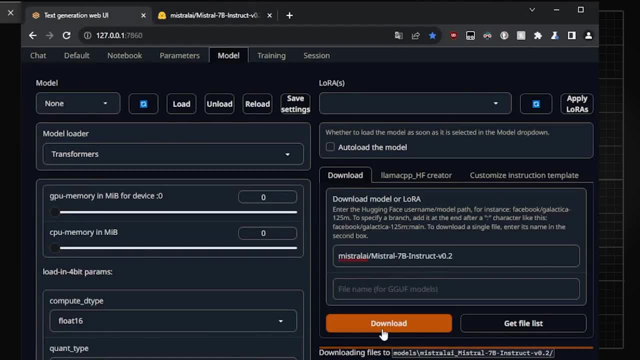 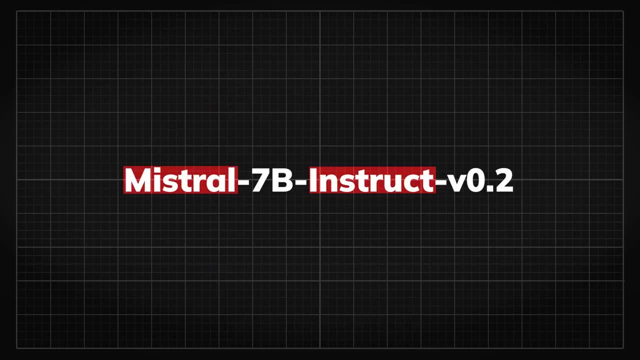 built-in downloader by copy and pasting the last two URL slugs. But if you don't have any models in mind, here's a list of models I recommend, along with their best usage, And besides their model names, it usually has their own version and a number followed by a, B, which means how many. 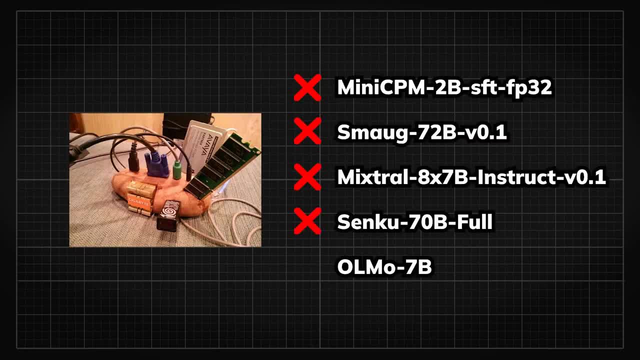 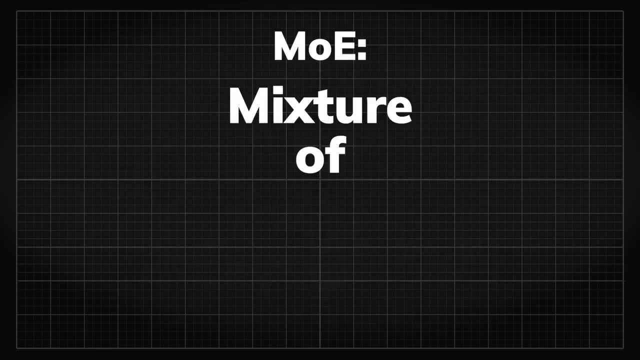 billion parameters the model has And it often acts as an indicator for you if you can run it on your GPU or not. But if it starts doing maths on its name or it says MOE, it means that it's a feature of Expert's model, which I explained in my previous video. you can check it out. 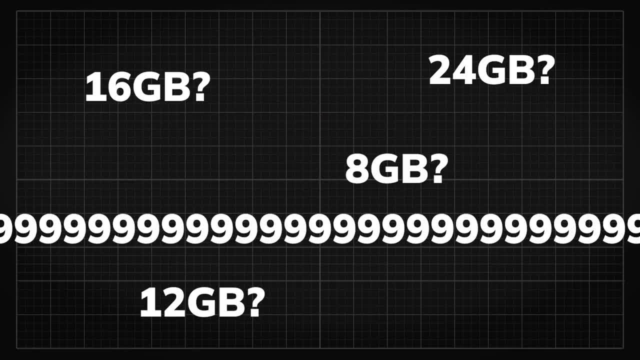 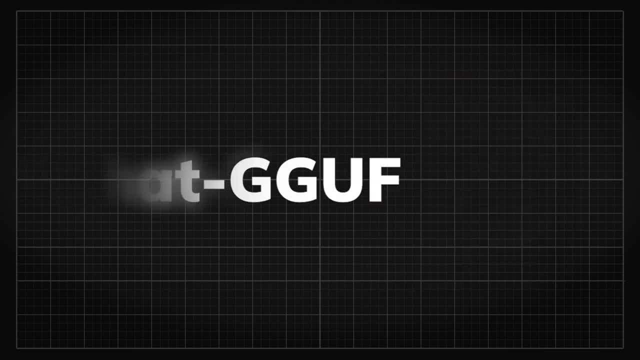 For a better approximation on how much VRAM you need for each model. you can also refer to these Hugging Face spaces. Sometimes you would see some other funny looking letters on their names too, like GGUF, AWQ, SafeTensors, EXL2, GPT-Q, but they are all. 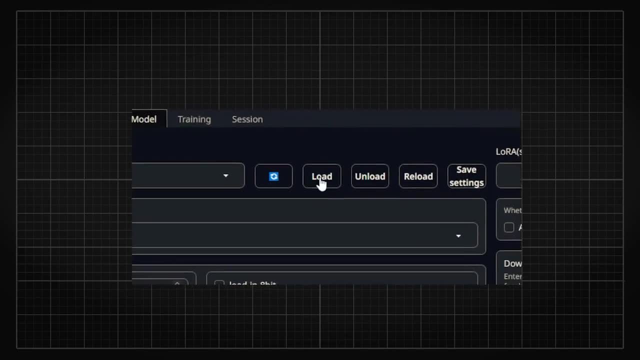 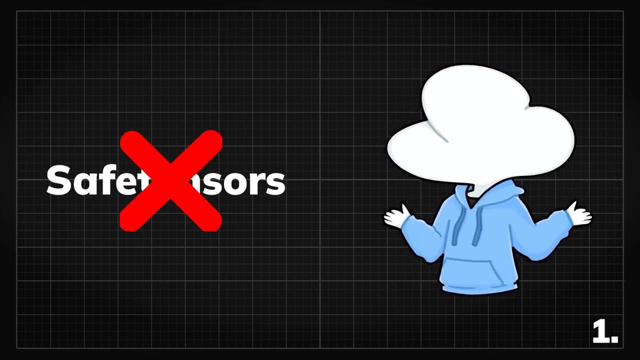 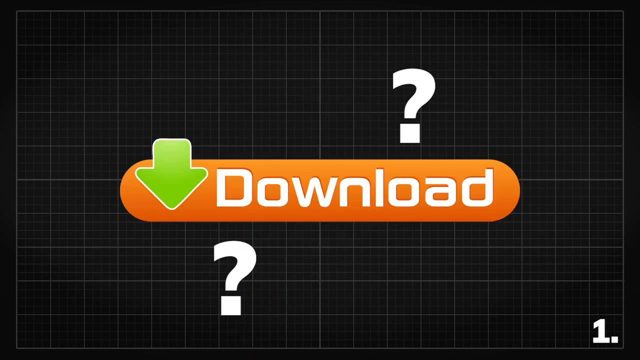 kind of meaningless until you start running your first model and encounters Runtime error- CUDA out of memory. Well, SafeTensors is technically unrelated to this, since it's just a secure file format that prevents people from adding such things to your PC when you load up a model from an unknown source. but others are different model formats. 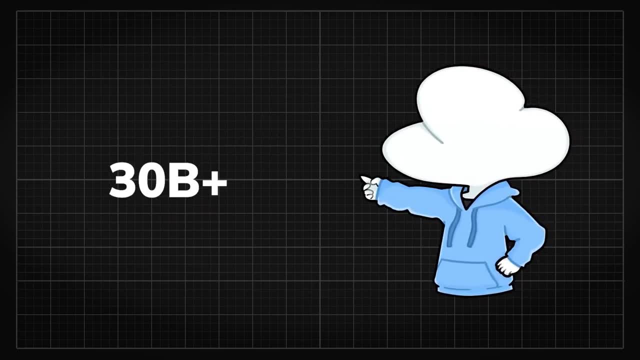 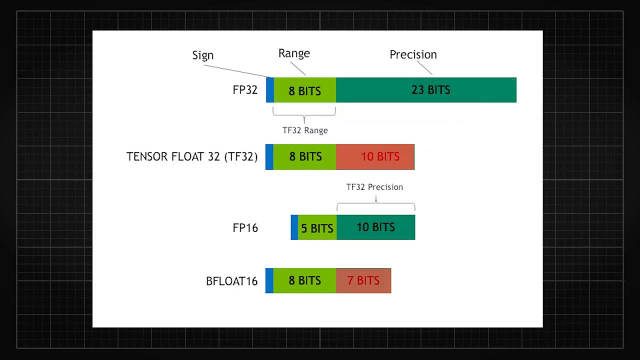 that potentially let you run them when you typically can, because of their large parameters count, And these formats achieve this by either shrinking down their precision or quantizing them, which is essentially reducing the number of bits used to represent a number that the model uses. 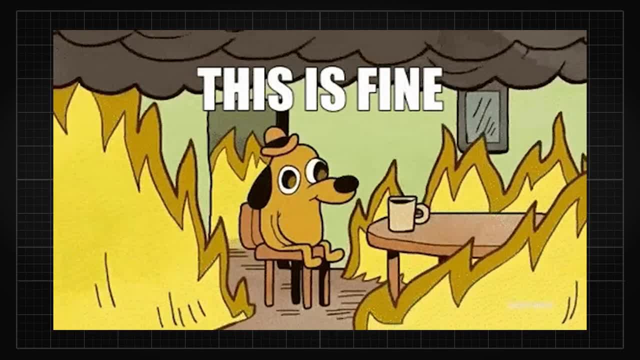 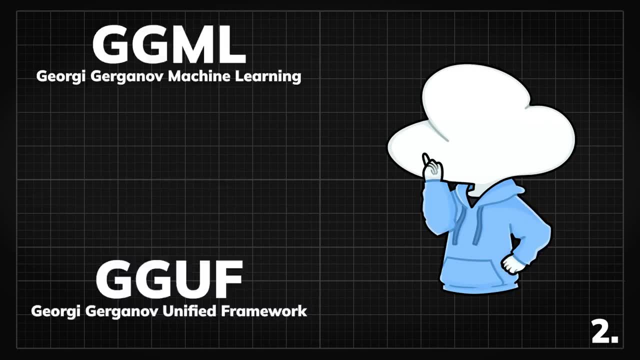 This would usually result in lobotomizing these models, but it's not as bad nowadays, since the loss isn't as noticeable when used on the better models. For the others, GGUF, a predecessor of GGML, is the file format in binary for models that supports a different quantization scheme. 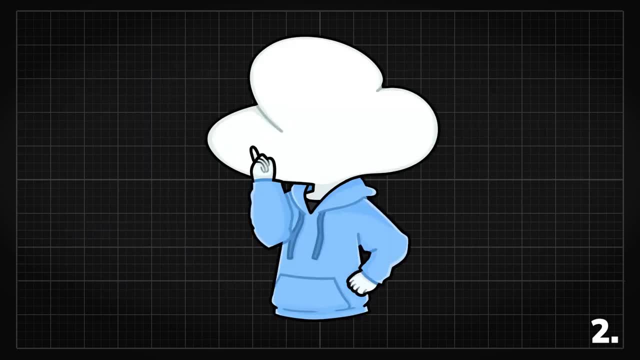 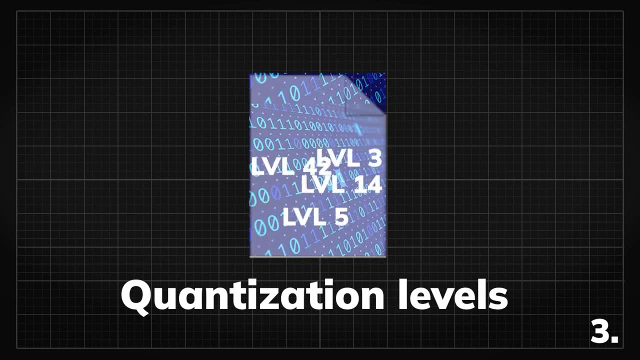 running on CPU and is contained within a single file, which most models are not. by the way, EXL2 is a format used by XLamaV2 which mixes quantization levels within a model to achieve an average bitrate between 2 and 8 bits per weight. It is the fastest optimization. 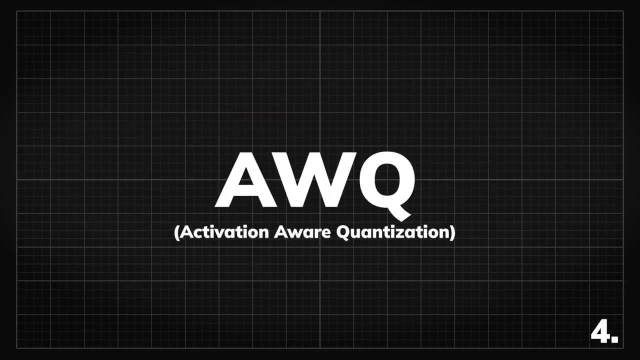 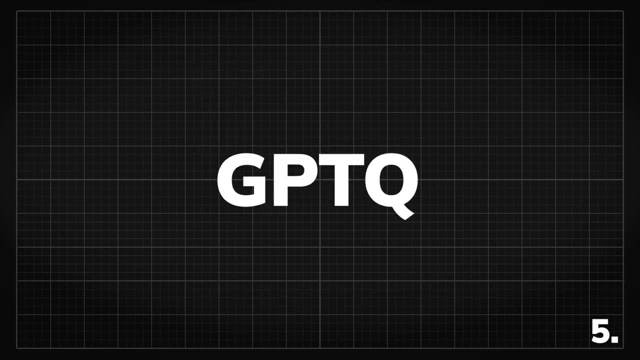 but only available on Nvidia GPUs. AWQ is a quantization method that sets smaller weights to 0 and round the rest to the nearest quantization threshold to reduce the model size. GPTQ is a layer-wise quantization algorithm which aims to minimize the error at the output, so it 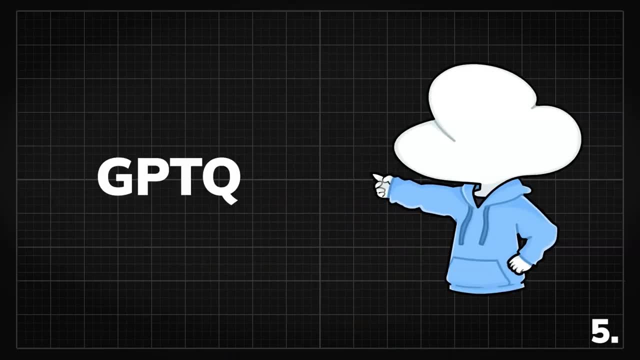 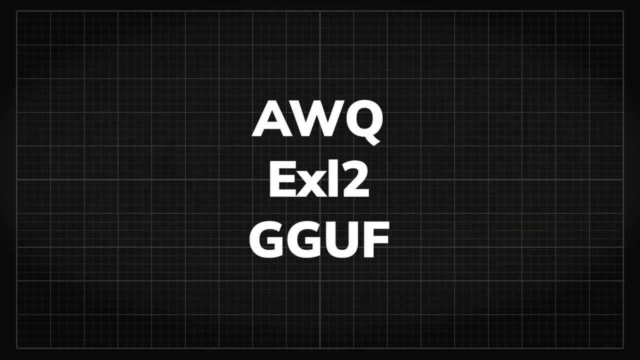 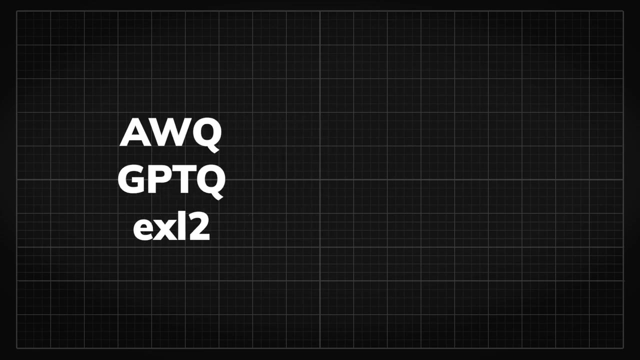 wouldn't blindly lobotomize itself. However, GPTQ and bits and bytes, which I have not mentioned, is not as practical for inference now, since AWQ, EXL2, and GGUF are just generally better, Apart from dot-safe tensors and dot-GGUF formats. these quantization methods are all making models. smaller after training, which almost always results in a lower quantization threshold. However, if you want to minimize the error at the output, you can minimize the error at the output. However, if you want to minimize the error at the output, you can minimize the error at the output. 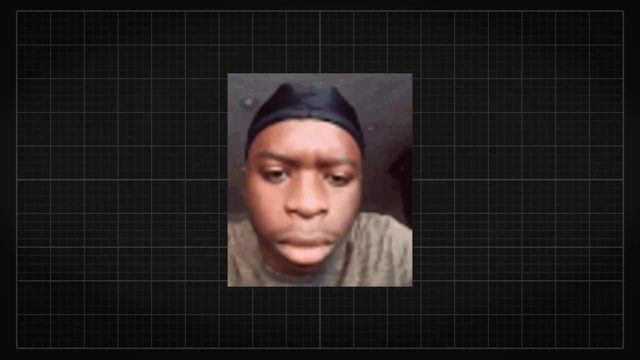 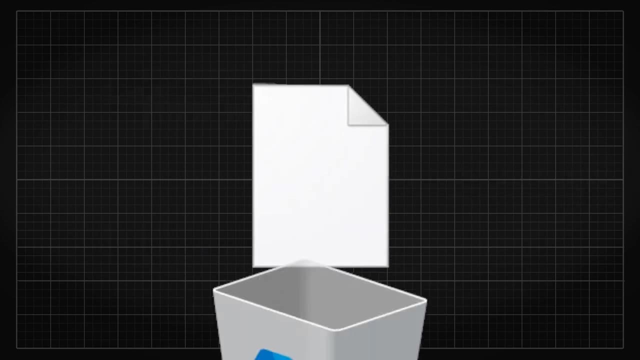 However, if you want to minimize the error at the output, you can minimize the error at the output, Because we still need to take into account context length, as it would also eat up your memory And not being able to provide a decent amount of context length would make the model kind of. 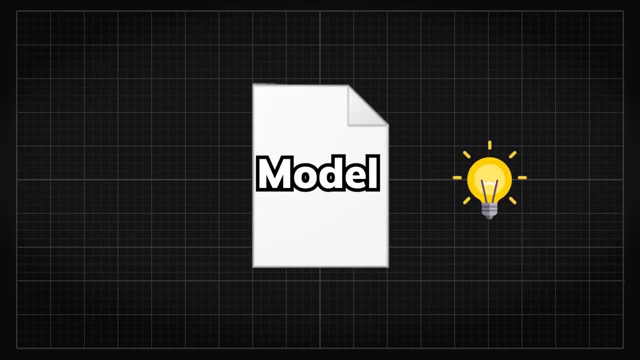 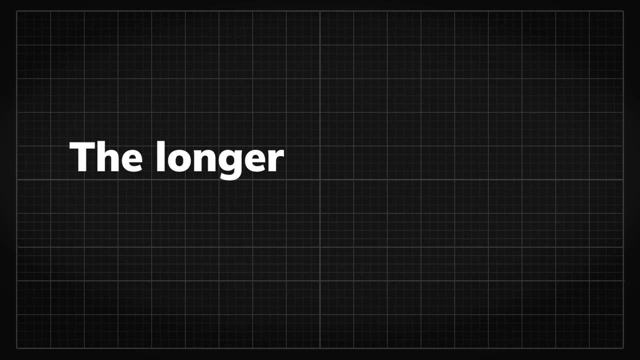 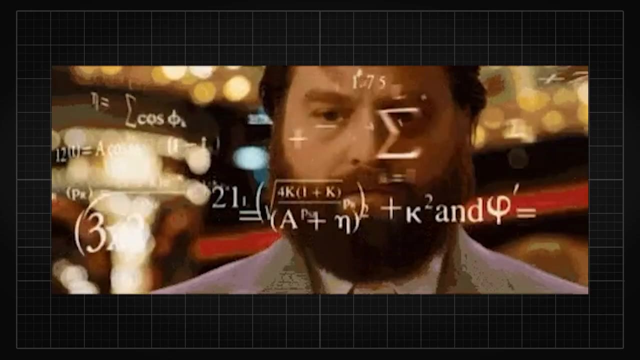 useless, since the model often needs context to solve your questions. For clarification, context length is everything which can be instructions, input prompts and conversation history, And the longer the context length a model has, the more information the AI can use to process your prompt with, like summarizing a paper or keeping track of what it generated in the 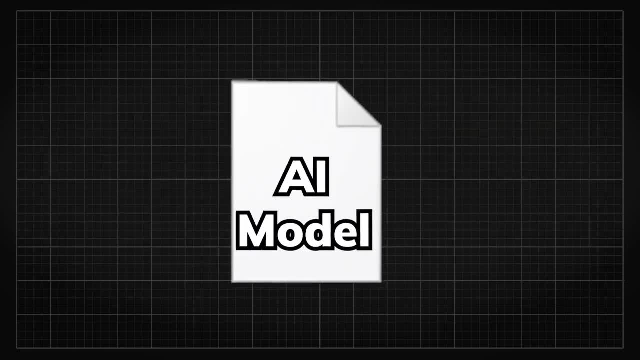 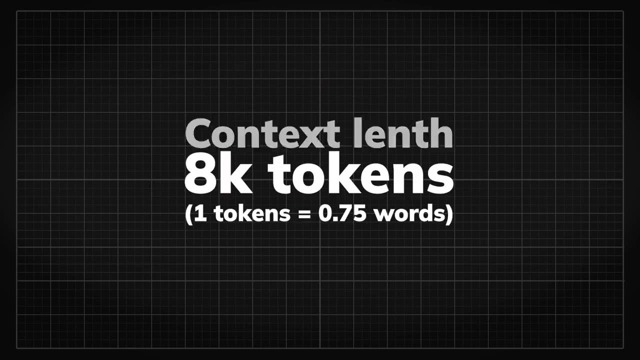 previous conversation. AI models don't save what you say to it, so instead you would need to provide history or data for it to use. For the precise technical details: 8,000 tokens. context length is usually around 4.5GB VRAM, but some models like Mixtro and DeepSeq can get VRAM usage. 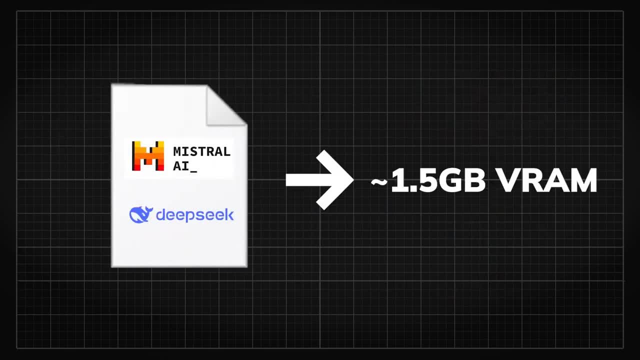 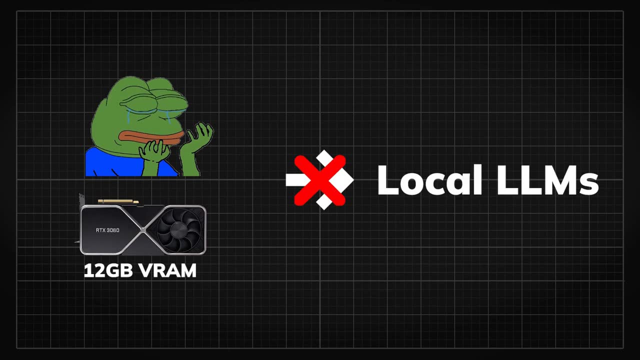 even smaller because they have GQA implemented, which is around 1.5GB for 8,000 tokens. So does that mean it is even more doomed for typical 12GB VRAM consumers to run local LLMs? Well, not quite. 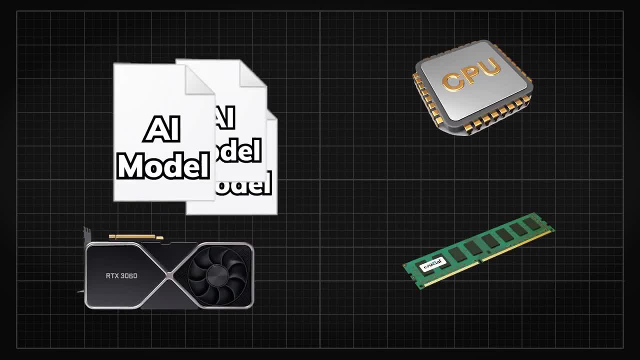 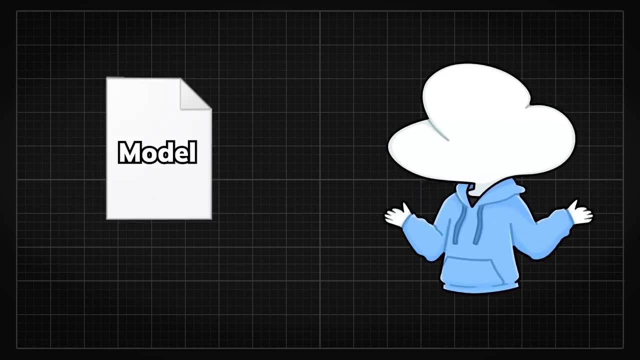 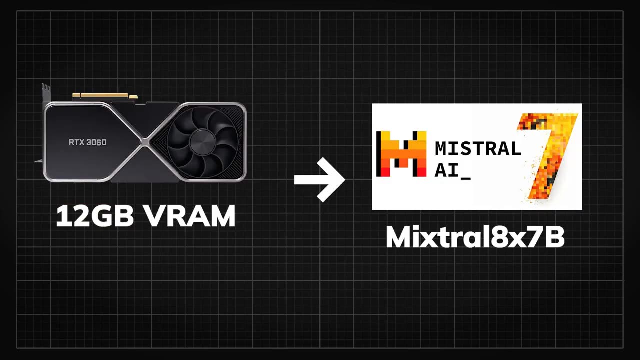 There is something called CPU offloading, which lets you offload models onto CPU and system RAM. It is a feature from Lama C++, the same people that made GGUF. so the model has to be in GGUF format to do this. But even a 12GB VRAM can run Mixtro AX7B, which is like 45 billion. 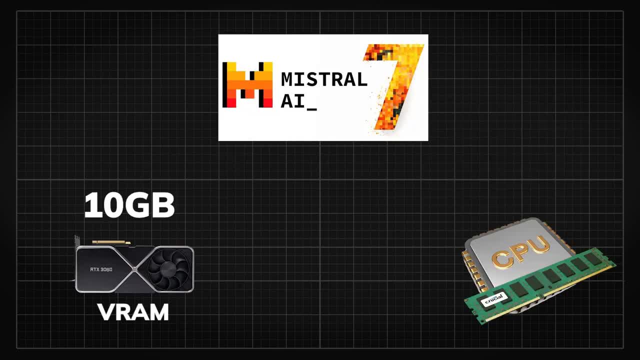 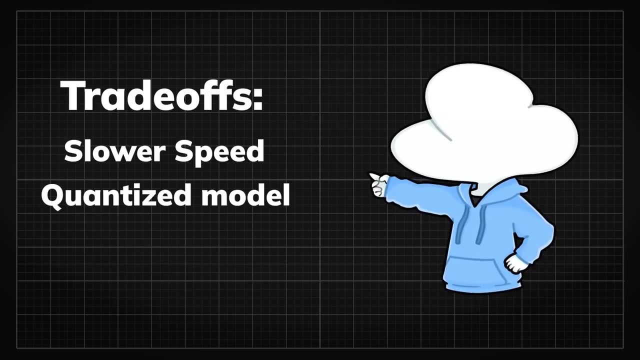 parameters in total by putting 10GB of the model in the VRAM, with 2GB for context and the rest handled by CPU and system RAM. While the trade-off is, of course, the speed and using the same CPU and system RAM, but with a higher CPU and system RAM, you would still get some pretty. 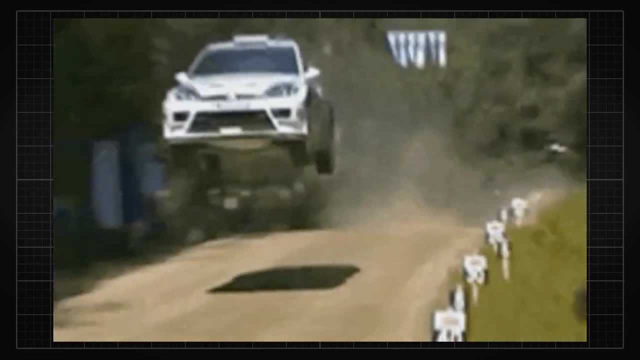 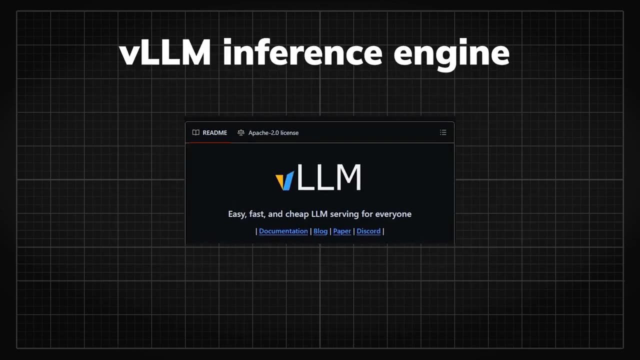 top-tier results for running locally for free. And if you do want to run it faster other than EXL2, there are other hardware acceleration frameworks like VLLM Inference Engine. that is great for server-side, where it handles parallel requests very well and increases. 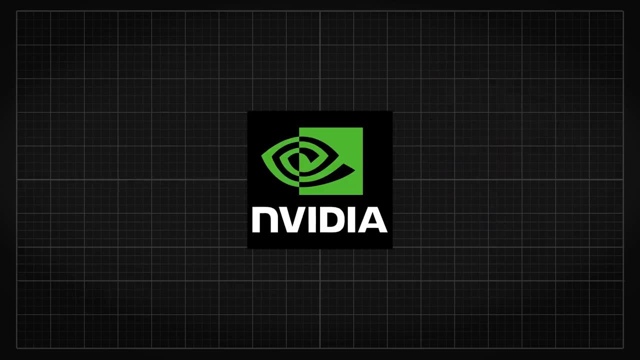 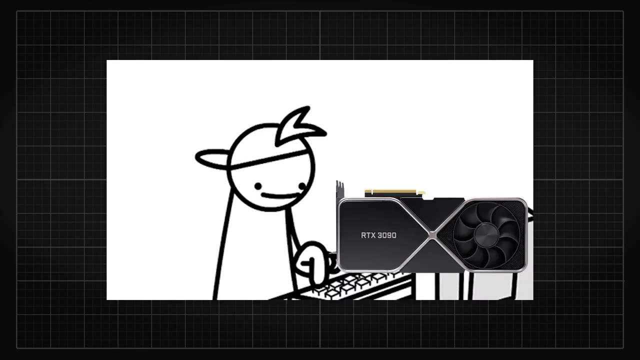 model speed by 24x compared to hugging face, And Nvidia is also offering Tensor RT LLMs that you can use for some popular models to increase inference by 4x with your RTX GPU. They also want to be able to run a lot faster, and they also recently released an app called Chat with RTX. 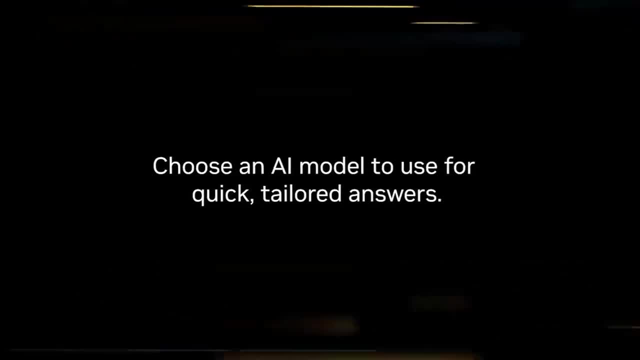 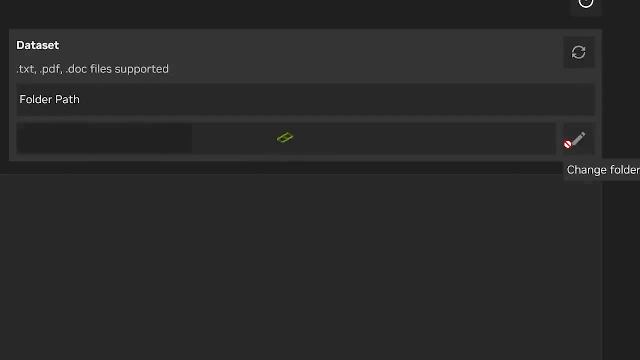 which is a local UI that can connect a model to your local documents and other data, so you can ask it to scan your documents without the need to upload it anywhere. Super good for privacy, if that's what you're looking for. It can also watch a YouTube video and answer questions about the. 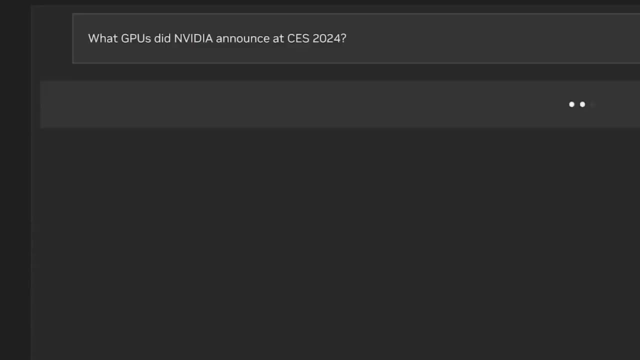 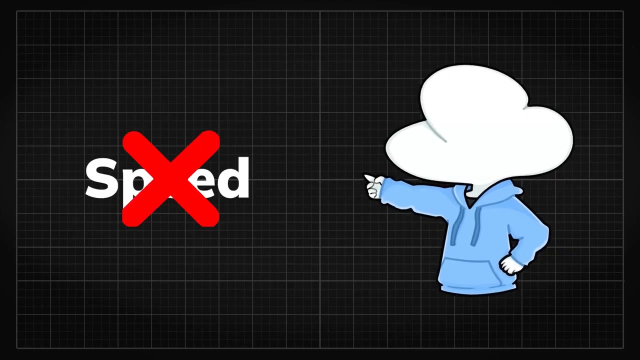 content of the video. so if you're too lazy to watch my videos or just need to revisit a few key points I've made, Chat with RTX can answer it easily for you. But if speed is not what you're looking for and you want the AI to do something with it, you can also use the app called Chat. 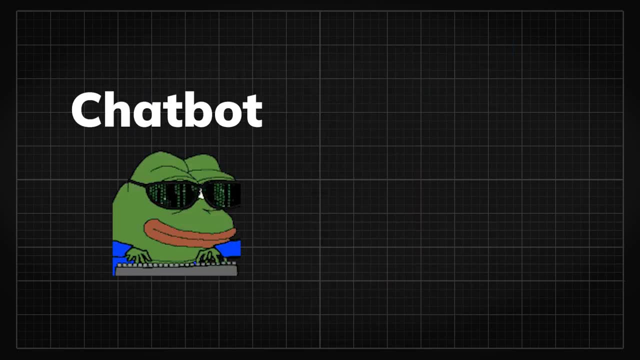 with RTX, which is a local UI that can connect a model to your local documents and other data so you can ask it to scan your documents and answer questions about the content of the video. Like becoming a chatbot that teaches you how to code, or becoming a tech support for. 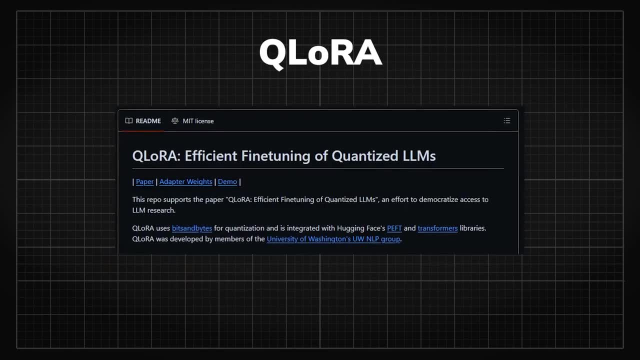 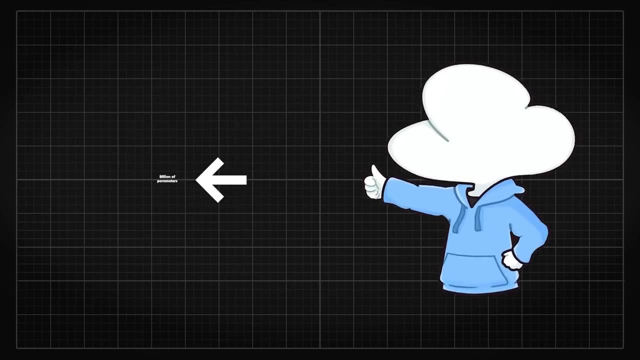 grandparents. this is where fine tuning comes in. Qlora is the current best way to fine tune a model, as it doesn't need to train the whole billion parameters model and instead only a fraction of them. Besides, no one really fine tunes the entire model as it is pretty inefficient and you 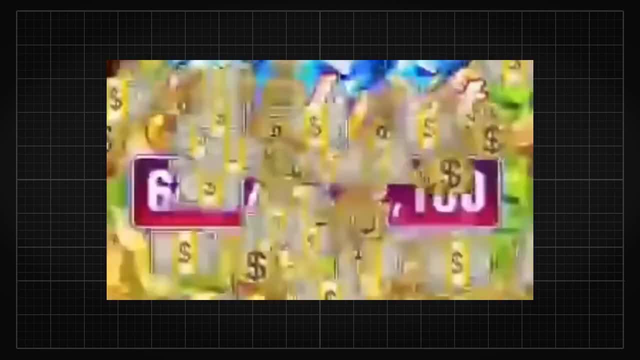 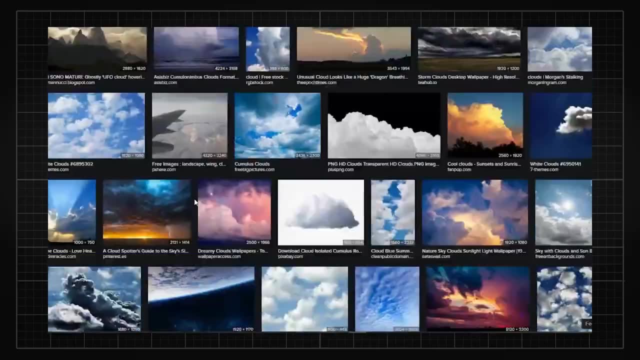 probably need to spend a quarter of a million just to train it for like a month. But before you start fine tuning it, remember the golden rule in AI: garbage in, garbage out. If the training data is badly organized, the result would be trash The model that you choose to. 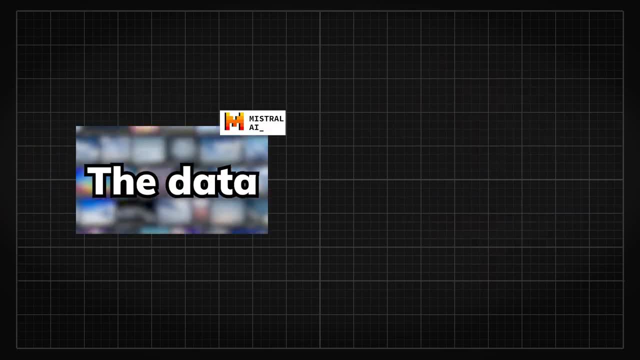 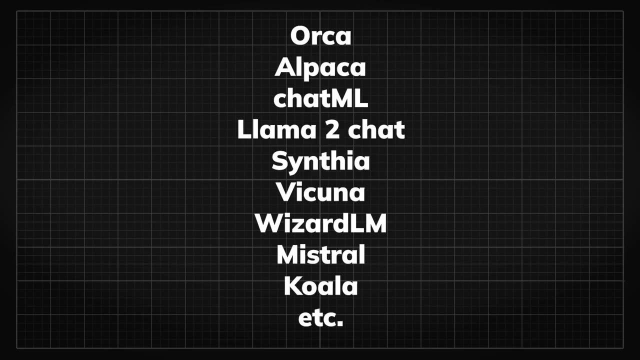 fine tune has to be a good fit for what you want it to do too. The dataset for fine tuning usually needs to follow the original dataset's format that was used to train the model you are fine tuning on. There are currently a lot of different formats, and because the data formatting is how instruction 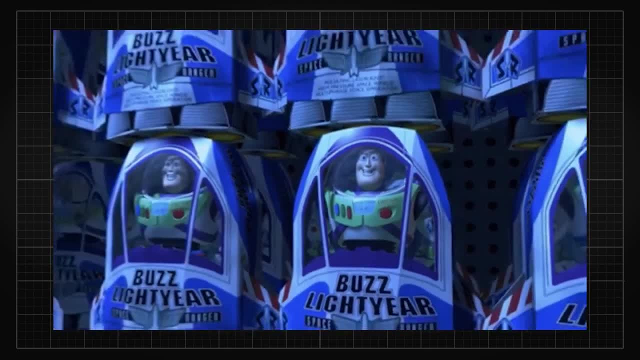 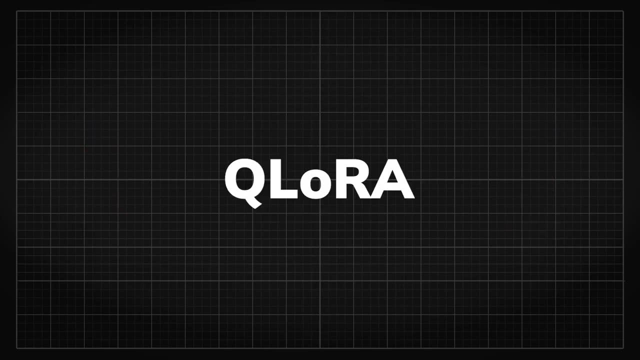 Q&A and dialog AI models are made, so to reproduce something of similar format, it's necessary to choose one correctly. There are other fine tuning techniques which have less capabilities than Qlora. however, they mostly serve a different purpose too, like get it to generate answers that satisfy. 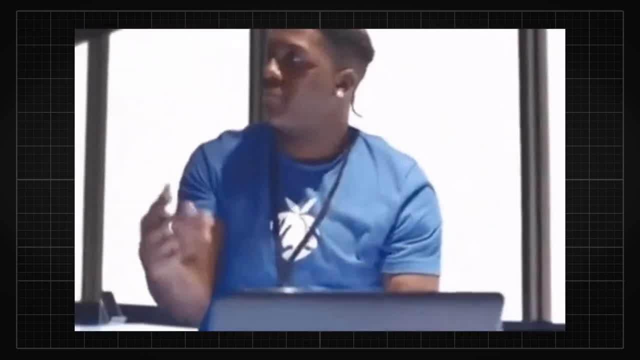 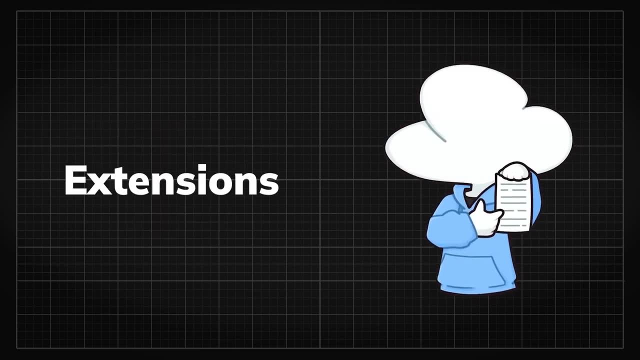 some moral guardrails or responses that are more preferred by humans. And yeah, these are roughly everything about running local LLMs in AI chatbots. There are also other extensions that you can use, like RAG, to hook up LLM with a database through Llama index, so you can do things like 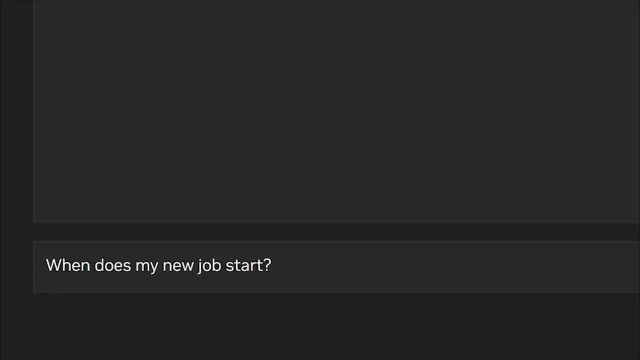 asking a model about some local files, just like it was demoed in chat with RTX, and even in a bigger scale. Or replacing GitHub CodePilot with continuedev using Qlora, Qlora, Qlora, Qlora, Qlora, Qlora. 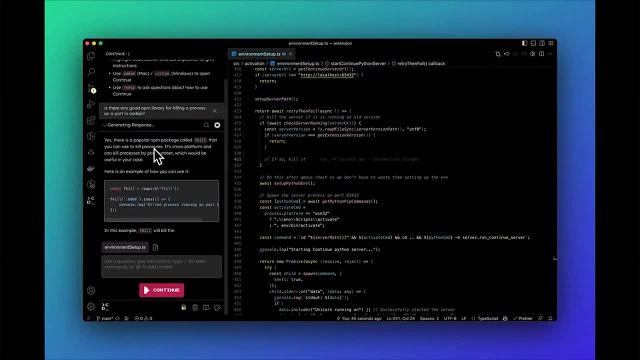 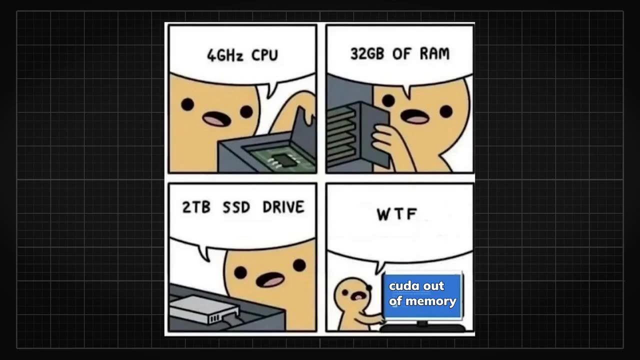 Qloradev using your local models, which would save you some more bucks. Running local LLMs may just be the peak of money saving in this age of AI without giving a performance, So maybe this is where you start your min-maxing journey in AI and run local models that will save you extra 20. 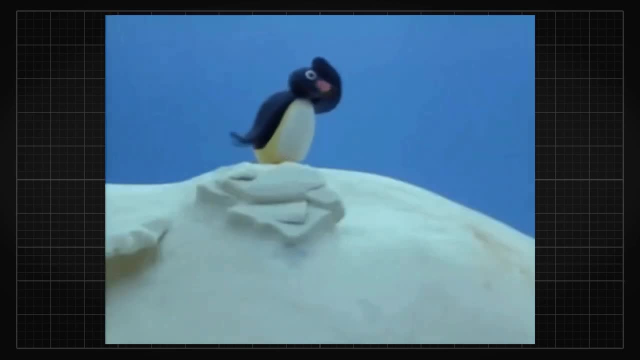 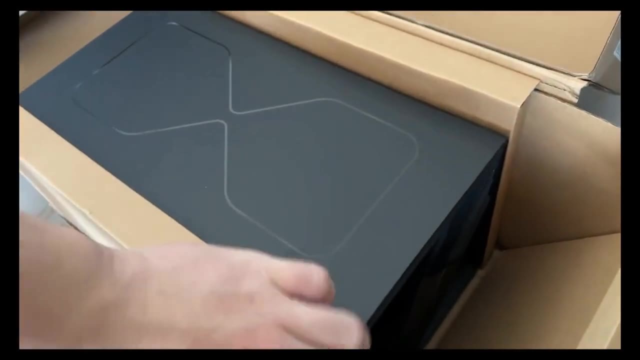 bucks during this hiring freeze, But if you are looking for more GPUs to run local models faster, Nvidia actually sent me an RTX 4080 Super to giveaway to you guys. And look at this bad boy. I'll probably not open this box, so whoever gets this can still enjoy the thrill of